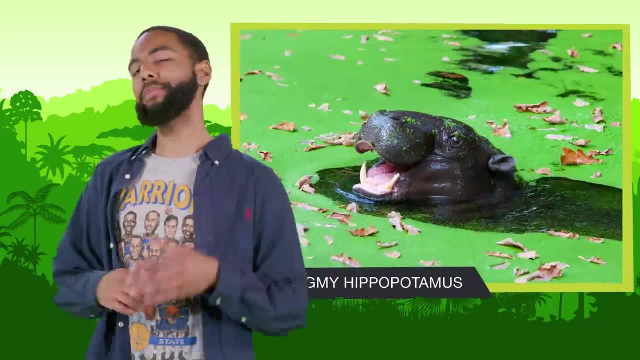 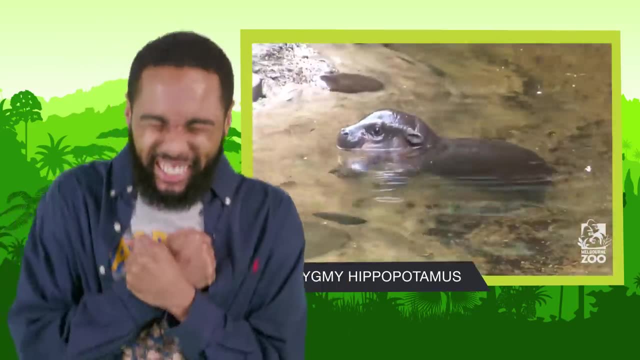 Meet the pygmy hippo. They live in Africa and they are too stinking cute, Like this little one. Oh my god, look how adorable he is. Too bad, these guys are dying out. Yep, they're in danger, There's. only about two or three thousand of them left in the wild, Mainly because you guessed it. as usual, humans are screwing something up. We're clear-cutting and logging their habitat. If they all die, the species will be gone forever. In a word, extinct. 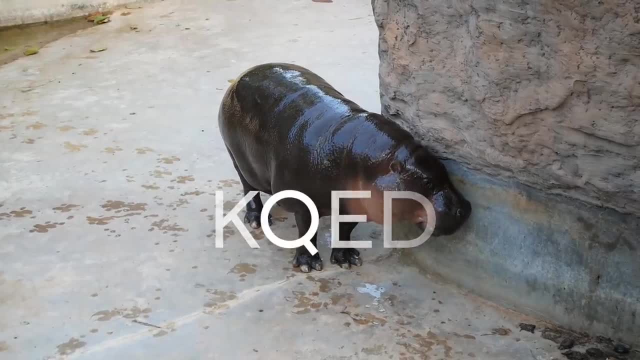 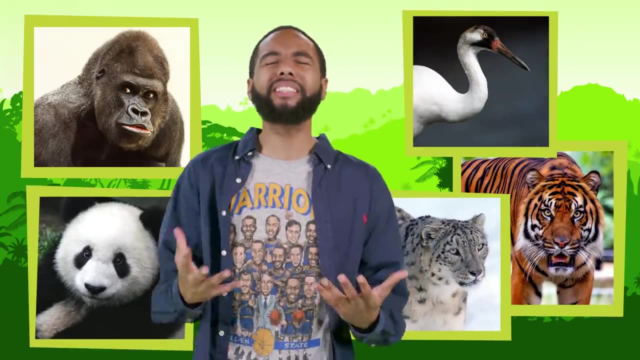 The pygmy hippo story isn't unique. There are lots of endangered species that environmentalists have been urging, imploring, just begging us to protect for years. They use all kinds of different tactics. They pull on our heartstrings and show us how cute and sad. 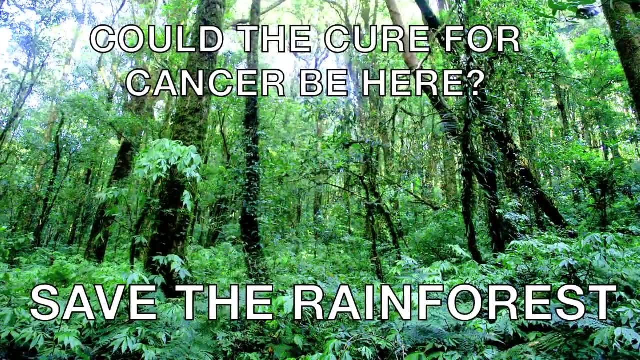 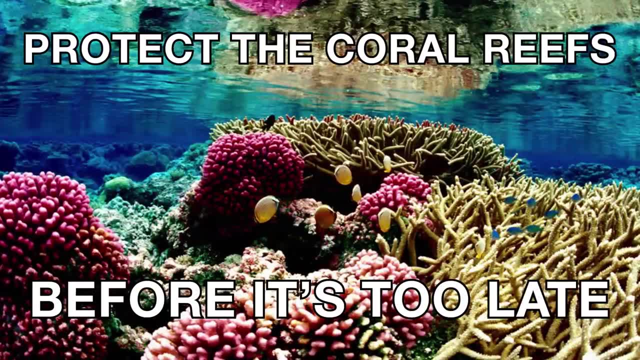 these little animals are. They appeal to our fears- Stop clear-cutting rainforest. one of those plants might cure cancer. And they tap into our selfish side, Like: if you don't save the coral reefs, you'll never be able to see these majestic places in person. 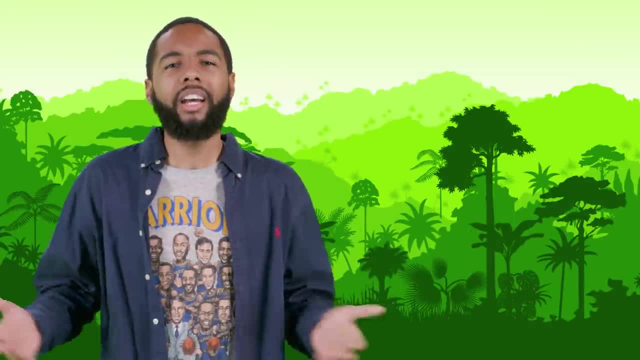 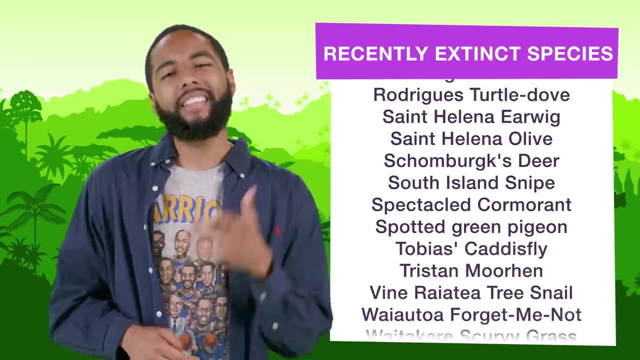 and take the perfect selfie, But despite all this, species go extinct all the time. Check out this giant list of extinct species, like the Caribbean monk seal, the Yangtze river dolphin and the St Helena earwig. So why should we care if a species goes extinct? I mean, does anyone really miss? 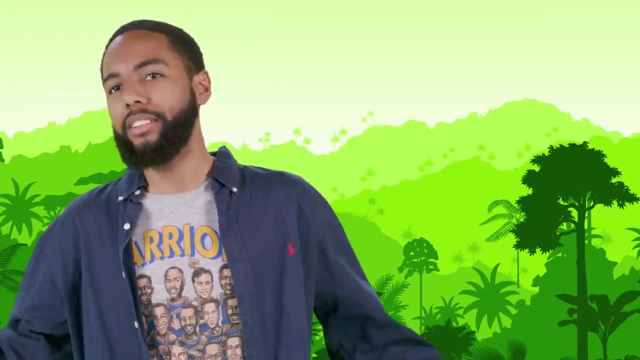 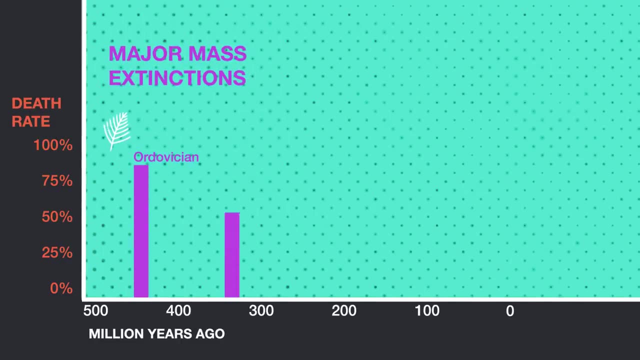 the St Helena earwig. Wait, what's an earwig Lauren? Oh, that, Okay. so throughout Earth's history, scientists know of five mass extinctions. This is when a ton of life on Earth got wiped out. This happened about 65 million years ago, when the dinosaurs all died off. But scientists are 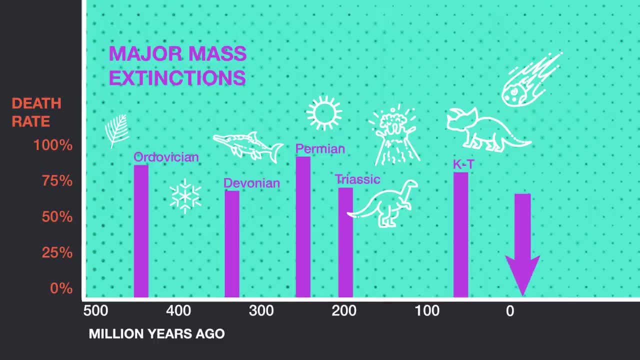 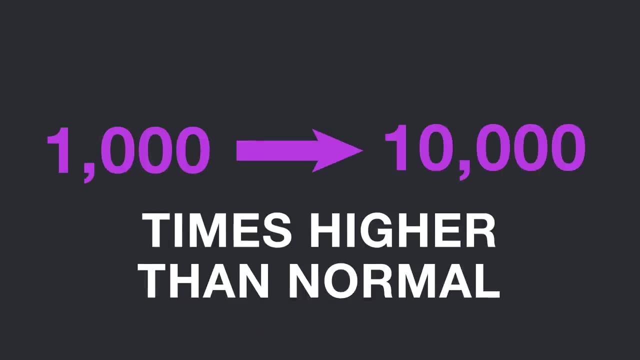 estimating. we're in the middle of the sixth mass extinction right now, where species are dying out at crazy high rates. Some estimates range from 1,000 to 10,000 times higher than normal, And for the most part we humans are to blame. We humans tend to destroy nature so we can live with all. 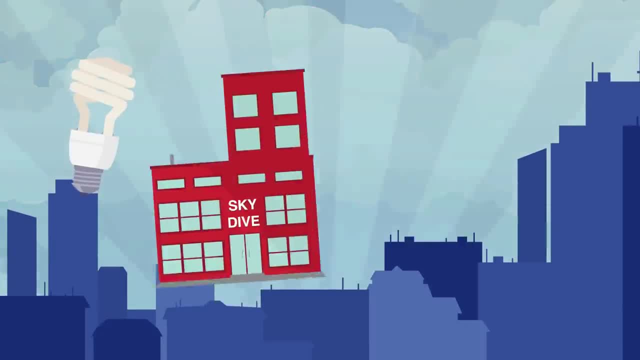 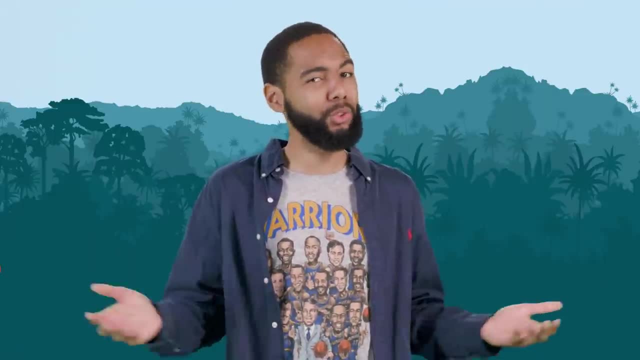 our luxurious, modern conveniences like electricity, indoor skydiving, food trucks and airplanes- I mean pretty much anything and everything awesome- And saving endangered species can be a huge pain and super expensive. So if you want to save your life, you need to save your life. 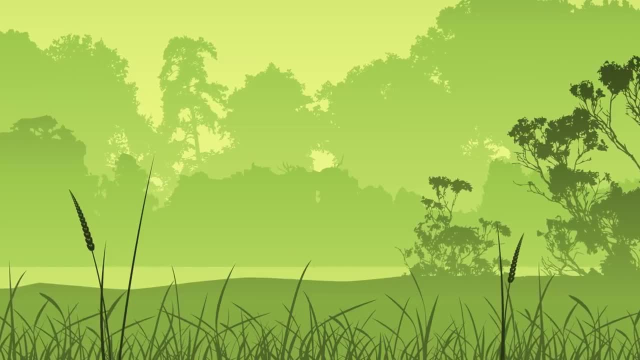 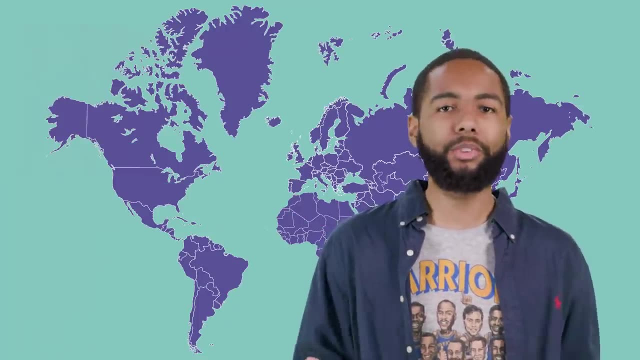 It can mean big sacrifices on our part, like you know, not building that awesome indoor skydiving building where these wetlands are. And it can be especially hard in developing countries. I mean, how do you tell people whose very livelihood depend on poaching or hunting endangered species to stop, Like in areas in Mexico where jobs are hard to come by. so people end up selling endangered sea turtle eggs, even at the risk of getting caught and spending nine years in prison. In a lot of places, this could be a life-or-death choice. 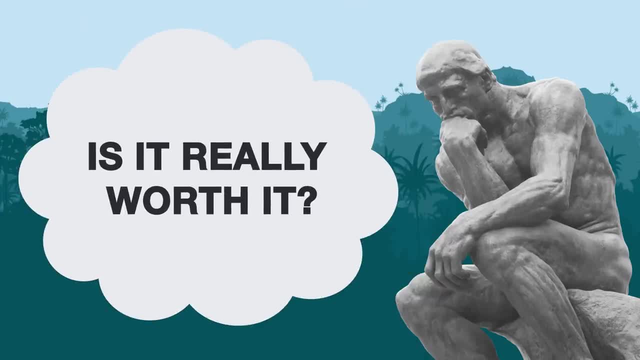 So is trying to save these endangered species really worth it? Well, there are a lot of people out there who are trying to save these endangered species, but they don't know how to do it. They don't know how to do it. They don't know how to do it. They don't know how to save. 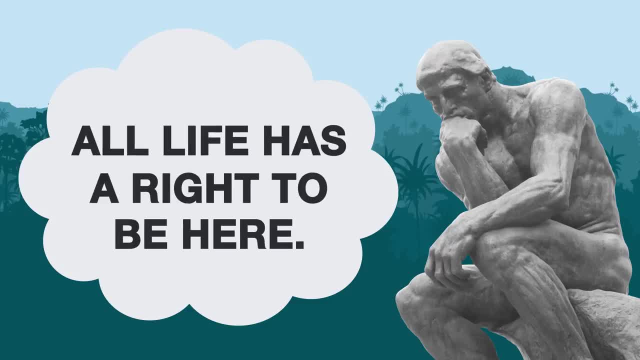 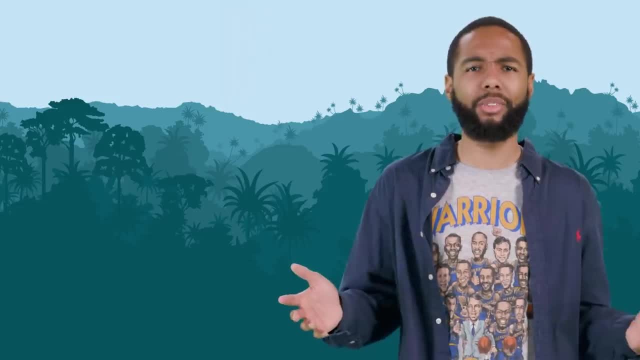 them. There are, of course, moral and ethical arguments to save species. like all, life has a right to be here, or that we owe it to our grandchildren to preserve species so that they can also see them in the wild. And let's be honest: when it comes to saving species, some of us 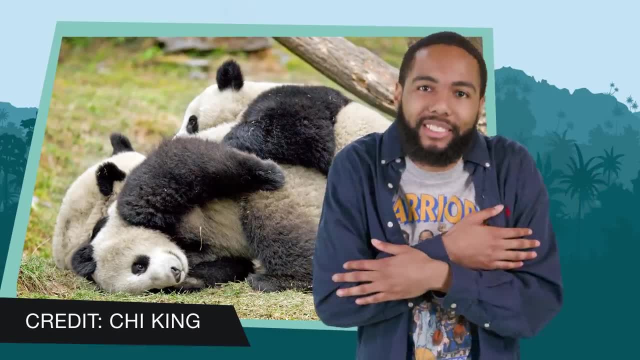 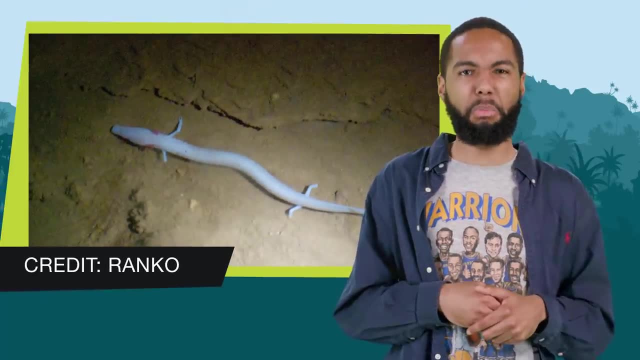 are more inclined to care about the oh-so-cute and adorable ones like these panda bears or these sand kittens, and it may be harder to get on board saving this weird-looking salamander called an om Ew, I mean, I'm not against saving it, but it is ugly. 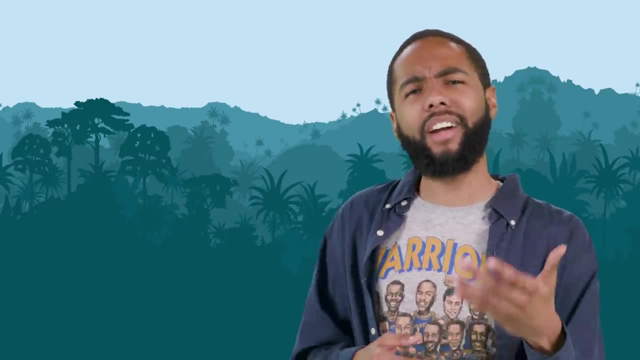 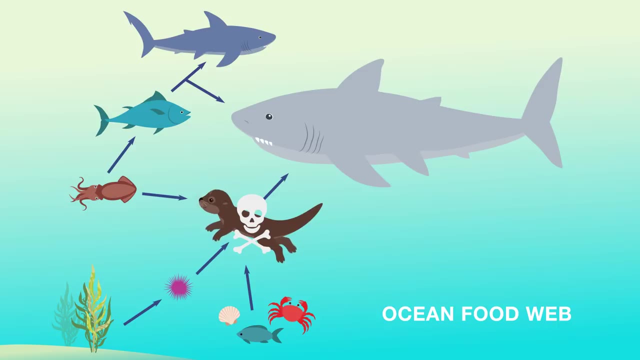 But more reasons aside, There are practical reasons we should care. Our very survival could depend on it. You see, living things in an ecosystem depend on each other, and the disappearance of one species can have big impacts on the whole thing, A lot like how a Jenga tower depends. 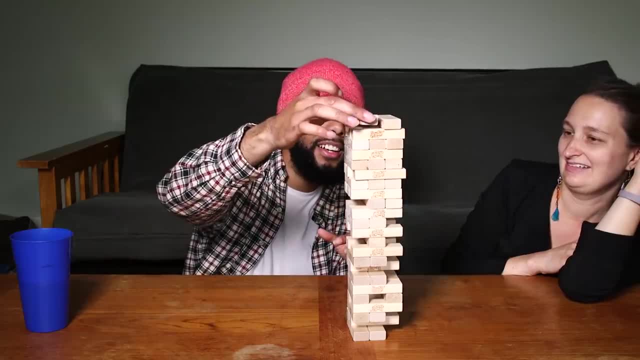 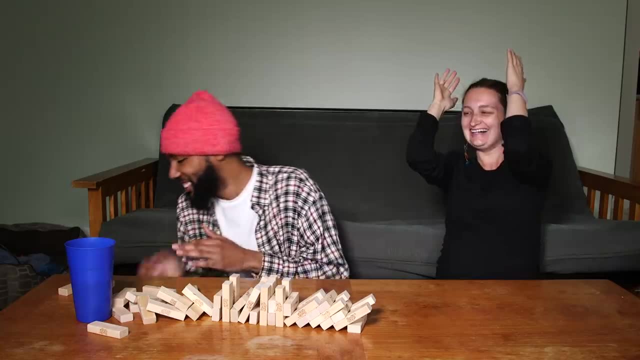 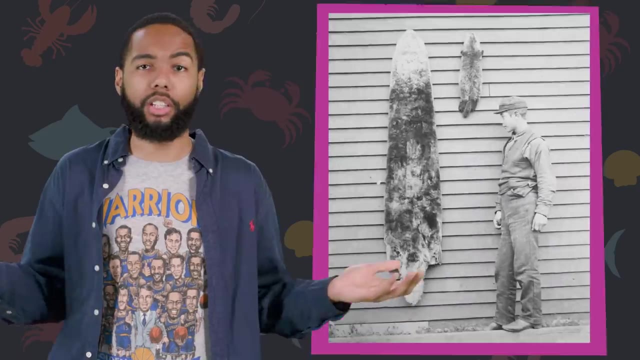 on each block and becomes more unstable as pieces are removed and rearranged. Take the cute, cuddly sea otter. They live in kelp forests and oceans and eat sea urchins. In the early 1900s they were hunted almost to extinction because they made luxurious 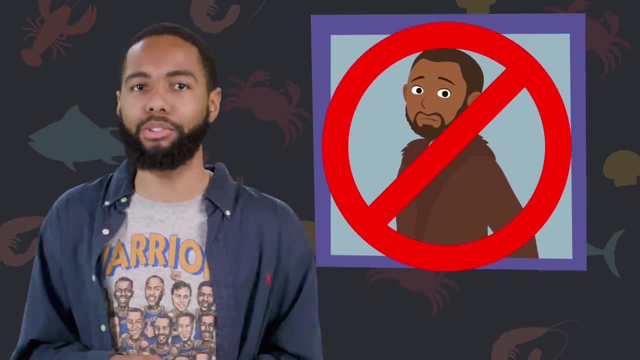 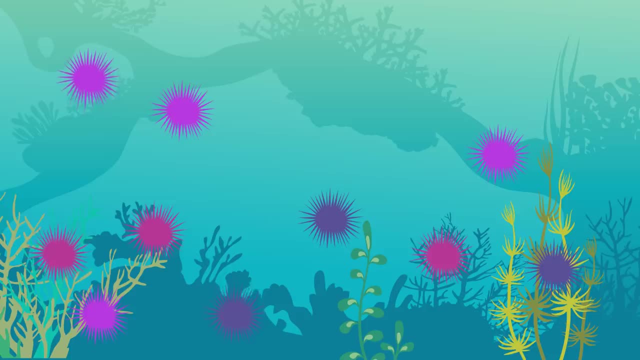 and fashionable fur coats. That is before wearing fur became a social taboo. And when the sea otter populations dropped, the sea urchin populations surged, eating up all the kelp and destroying the kelp forests. And if you're thinking so, what I've? 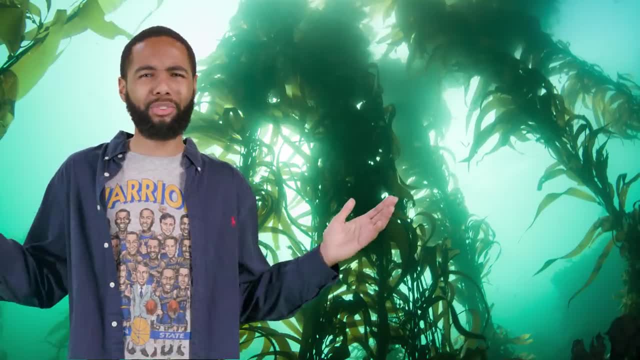 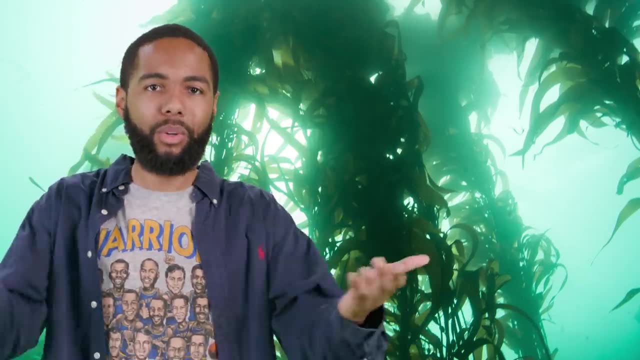 never even heard of a kelp forest. First of all, kelp forests are these crazy cool underwater forests made of these giant seaweed-type structures. and secondly, they are crucial to the overall health of the ocean and we benefit a lot from them. They provide habitat, food and water. They are also a source of food for the environment. They are also a source of searching for the best for the environment. They are also a source of food for the environment. They are also a source of food for the environment. They are. 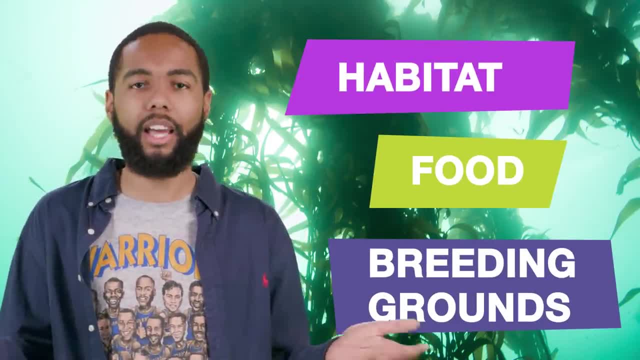 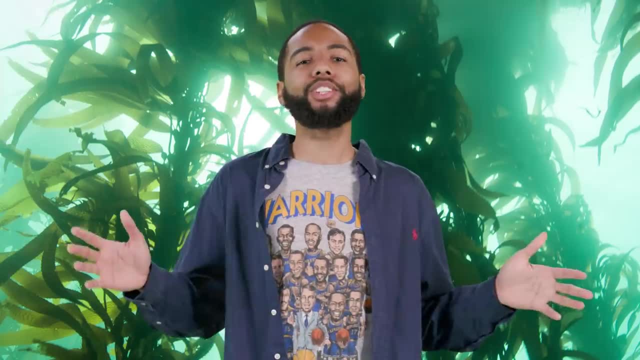 and breeding grounds for a lot of marine life, including some tasty seafoods you might like, like lobster, crab and rockfish. We're getting something to eat after this, right For sure. Kelp forests can also protect coastal areas from flooding due to storm surges. 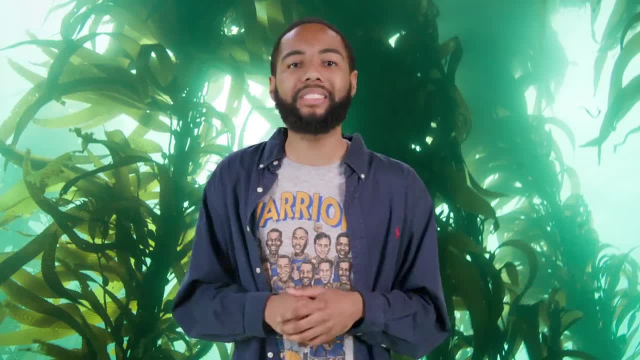 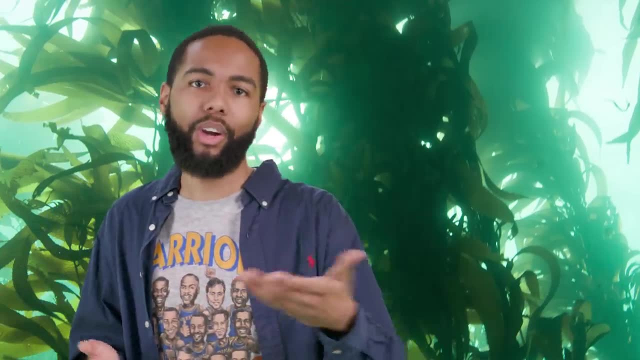 and they're made for some pretty cool scuba and snorkeling spots. Not to mention kelp is in a lot of beauty products like shampoo. The list goes on. So right about now you should be starting to feel sad about the sea urchins destroying this cool habitat.